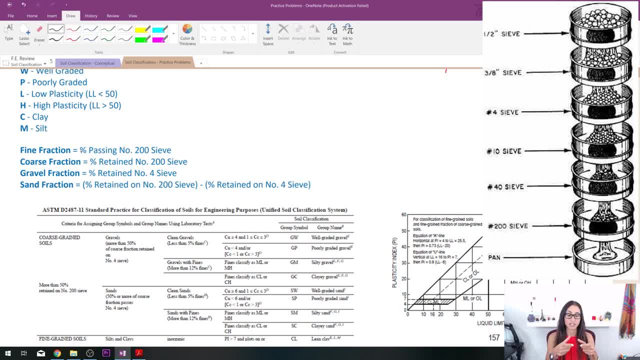 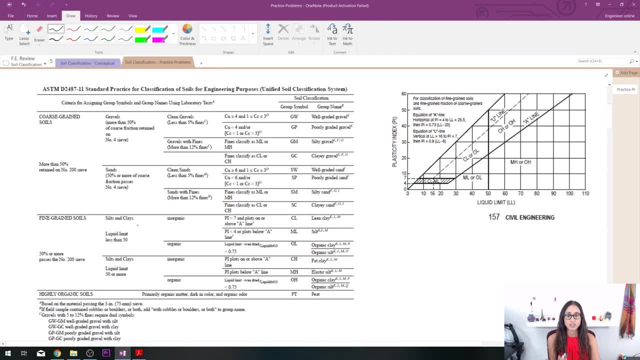 to determine the cent fraction. what we do is the percentage that is retained in C200 and we subtract it from the percentage retained on C4.. As I mentioned also in one of my previous videos, make sure that the NCES handbook you have it open as you're studying. 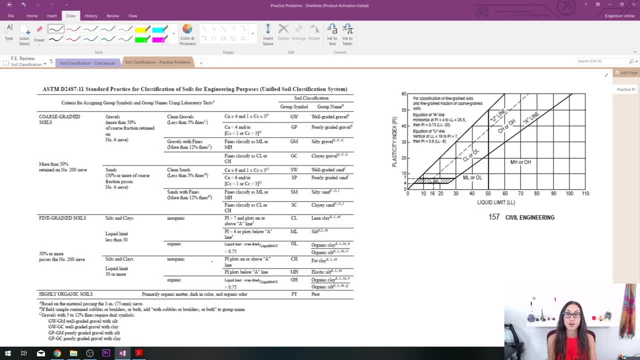 so that way you can locate all the equations and the tables, For instance this table- I actually got it from the NCES handbook, So this is on page 157.. We have the USCIS table and then here we have AASHTO table. 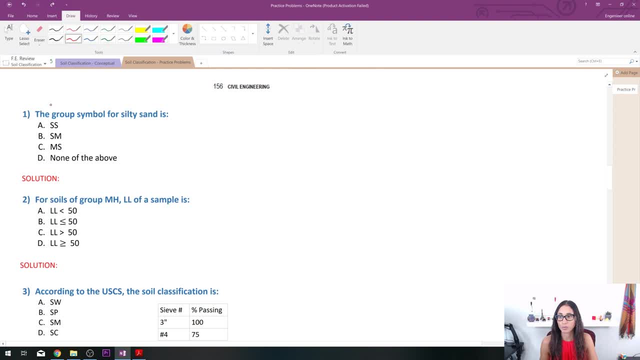 which is on page 156.. Okay, so let's start with problem number one. We have the group symbol for silty sand is SS, SM, MS or none of the above. So let me grab the handbook, here we go. 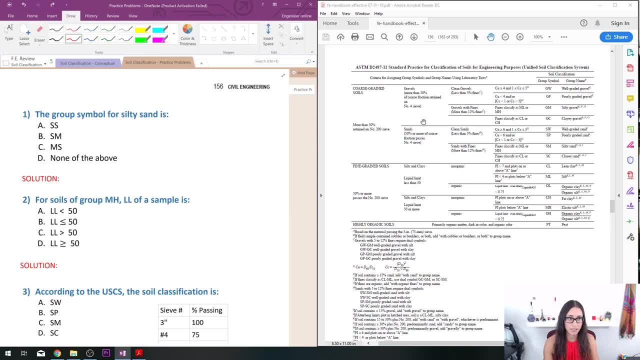 So this is the USCIS table. So if we look at the term here- silty sand- so we mentioned earlier that SILT is sand for M right. So already just looking at this you know it's gonna be either MS or SM right. 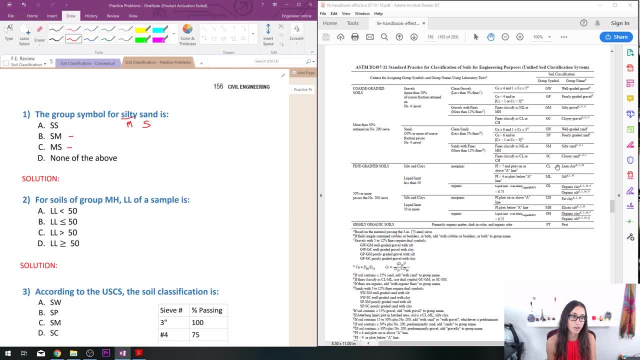 So in this case, what you do, you can just look at the table right here and then it already tells you. so there's basically no MS at all. There's only SM, which is silty sand. so that's your answer. 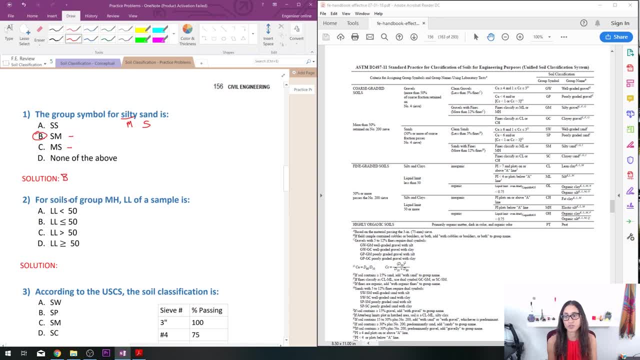 So it's gonna be SM. This is really easy question. The first two are really simple, just kind of a review, but then it gets. you know it's gonna be easy question. It gets more a little bit harder. Okay. so question number two. 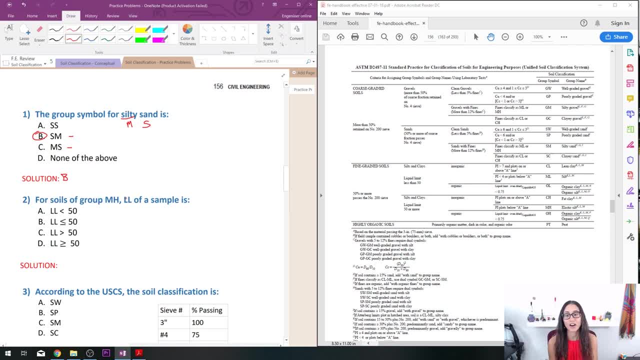 we have four soils of group MH. MH, the liquid limit of a sample is less than 50, less than or equal to 50,. greater than 50, or greater or equal to 50.. Okay, so again you do the same thing. 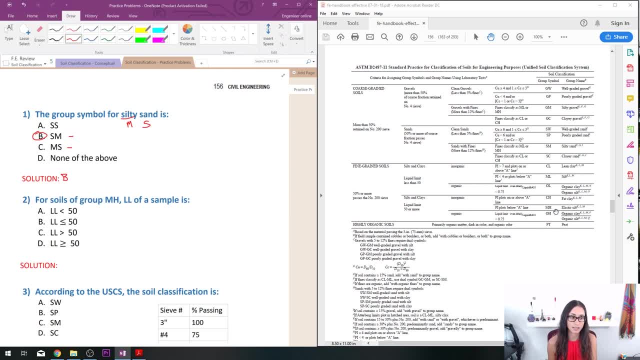 We go to the table, we look for MH, which is elastic silt, And then here you have your liquid limit, And so it says 50, you know 50,, 50. or more. so we know it's going to be greater, right? so we either have this one. 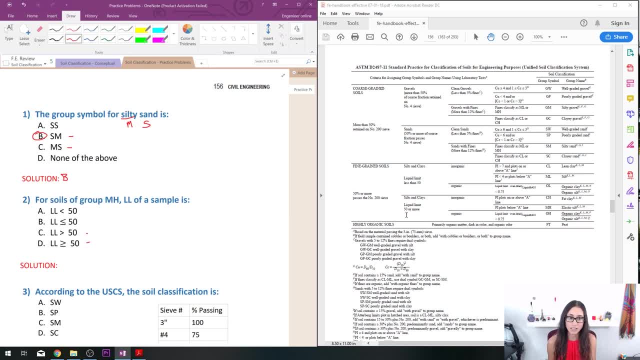 or this one. but then it says: here it says 50 or more, which means it's equals to 50 or greater. as for here it says less than 50, that means 49 and less. so 50 is not included. so which means, for our case and H, since it's here the 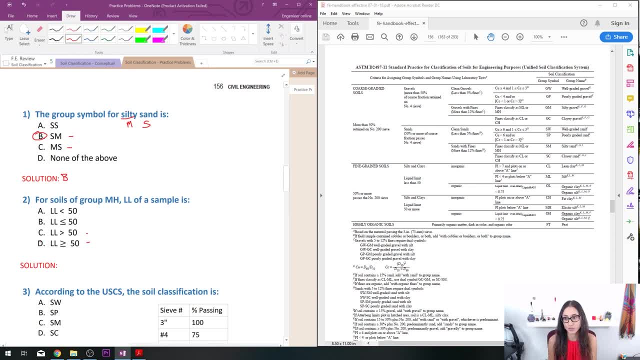 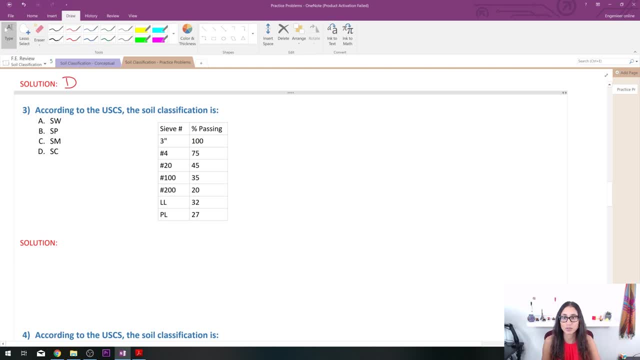 liquid limit has to be equal or greater than 50. so your answer has to be D. that's your answer. so question number three: according to the USCS, the soil classification is SW, SP, SM or SC. now the percentage, passing and sieve number are given to us. so let me pull out the handbook. here we go. first thing we're: 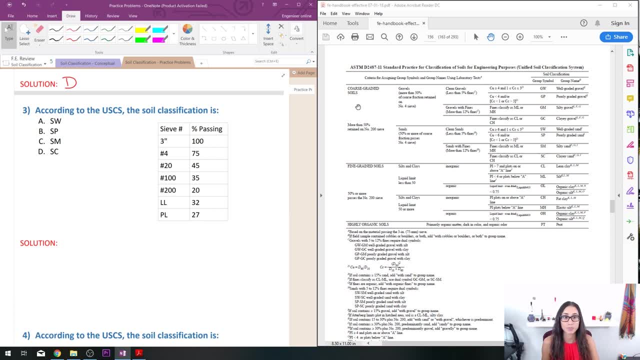 going to look at is the number 200 sieve, because that will classify our soil in terms of the percentage passing, and the number 200 sieve because that will is if it's coarse or if it's fine. so note also that if you get, let's say, 50%, 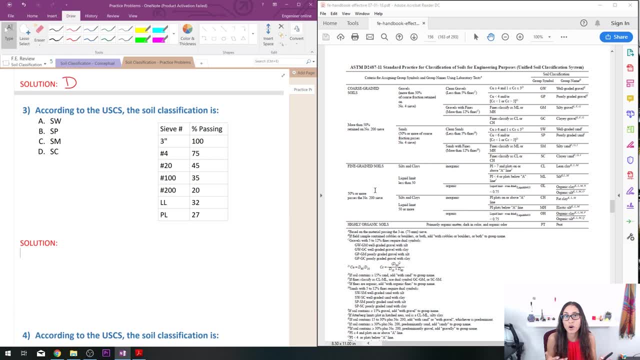 exactly it was giving to you. that numbers: 200 sieves is 50%. now you have to keep in mind that will be classified as fine if you get 49 or less. that would be coarse grained. so make sure for- and when I say 49 less, I mean 49% passes. 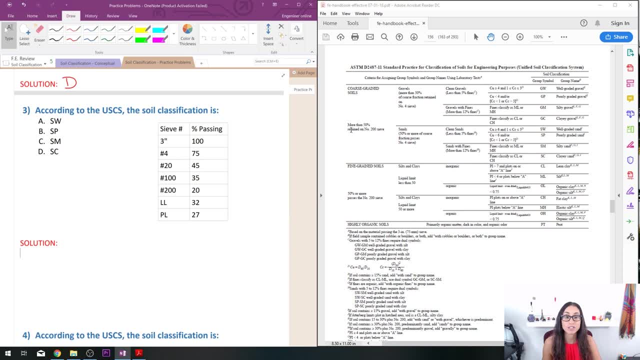 sieve 200. now also pay attention to these terms. here it's used to retain, but then here they use passes. so just be careful with the terms and with greater or less, so you're not confused, okay so? so let's look at the our 200, so our number 200 sieve we have. 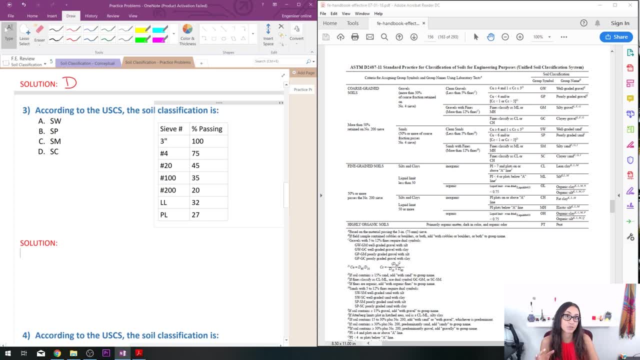 20% passing, which also can mean 80%. that is retained. so I have more than 50% retained, right? let me write it down, just so it's clear. so this can also mean that 80%. I just did 100 minus 20, right, because if its 80 is, 20 is being a past. 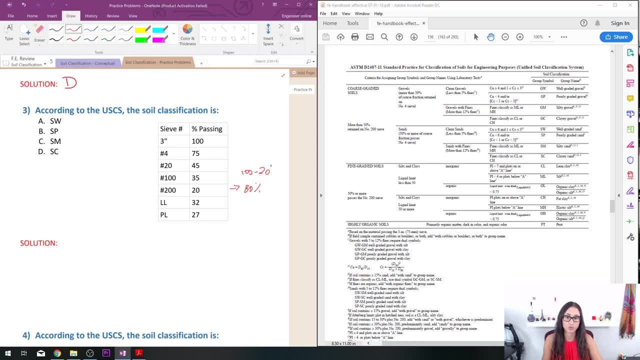 that means 80 of it. it was retained, so 80% retained. so if I have 80% retained I can already classify my soil as course. so I have coarse grained. that's because I 80% retained for sieve 200. okay. so the next thing we're going to look at is: 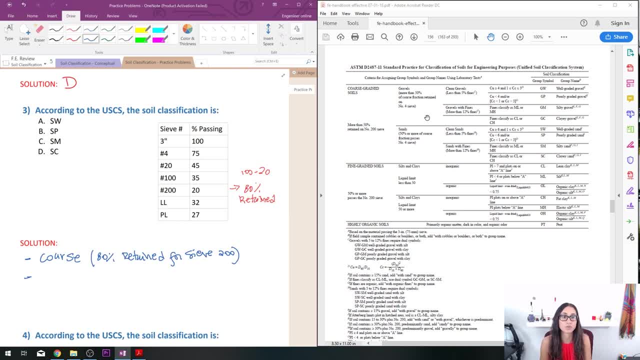 sieve number four. that's because it's going to define or classify our soil, either gravel or sand. so for my number four I have 75%. that passes sieve number four. here more than 50% is retained. and then here I have 50% or 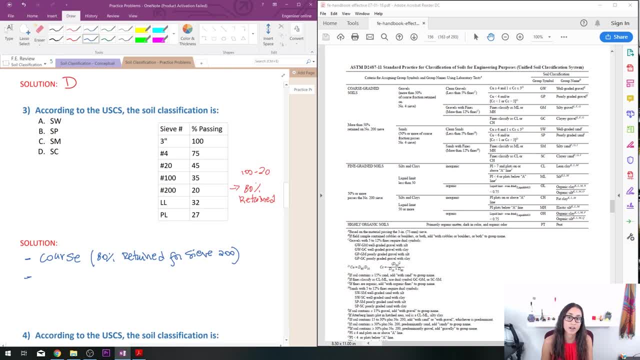 more passes. sieve number four. so 75 passes. so I'm going to go, so I have sand because I have more than 50%. that is, that's passing sieve number four. okay, so we're going to write here sand. so I have coarse, and then we said it's classified. 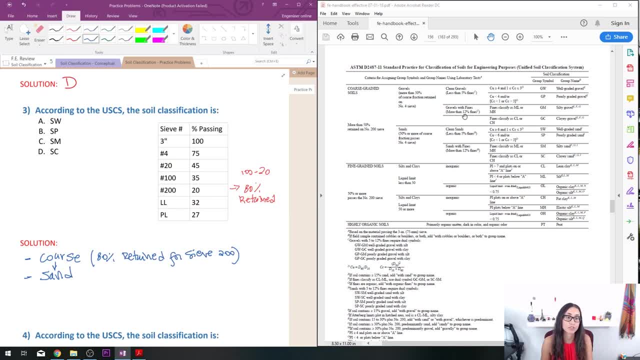 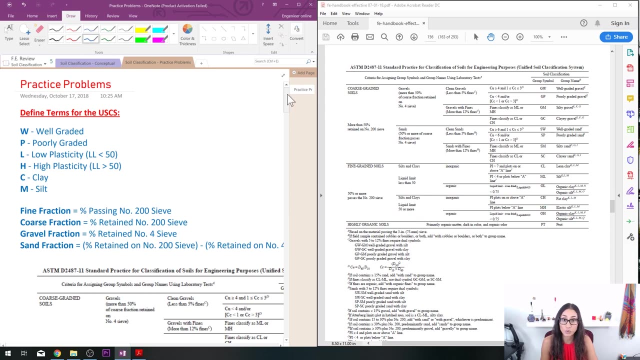 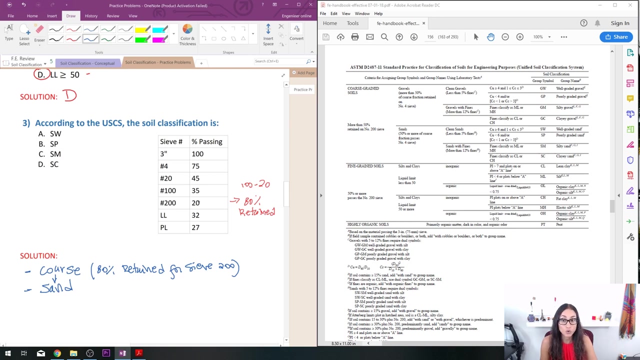 as sand. now, after that, we're going to need to define either: is it clean sand or sands with fines? we talked about that earlier. we defined it here. we said that the fine fraction is the percentage passing. sieve 200, correct? that means my percentage passing here for number 200 is equal to 20, which is also my fine fraction. so this is also my. 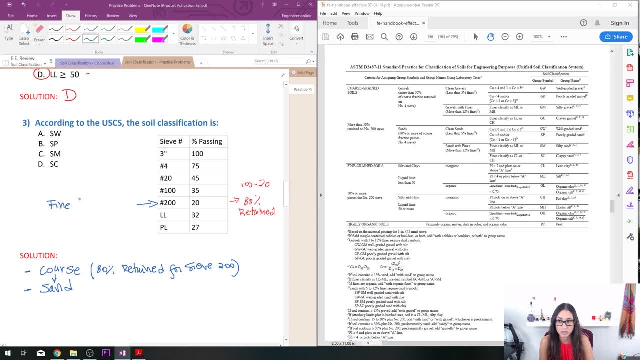 fine fraction which equals to 20%. so that means, looking at the graph here, more than 12% fine I have. so this classifies my soil as sand with with fines. so that's gonna be my next step. so I classified it so far as sand with fines because my, because I. 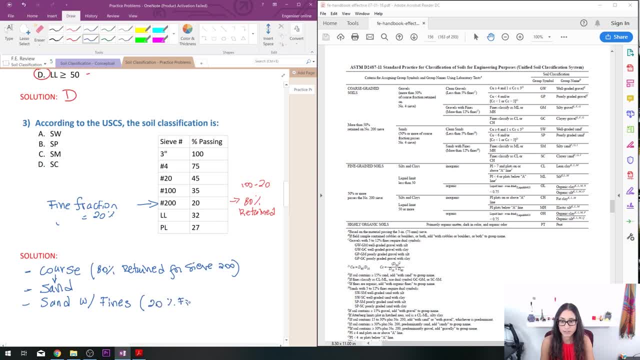 have 20% of fines. as for here we said I have 75% of c4. okay, so after that, which is the last step. so here we already know it's going to be either SM or SC, so either this one or this one. okay, so to to determine which one this one is a. 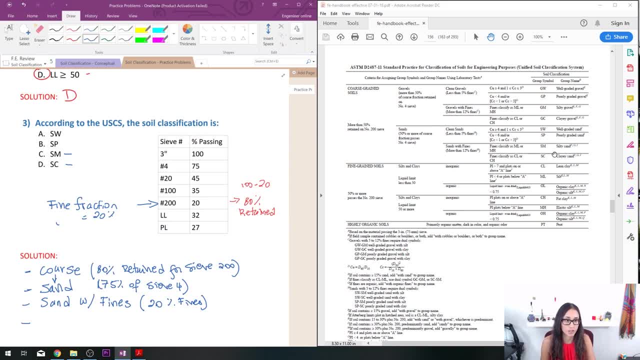 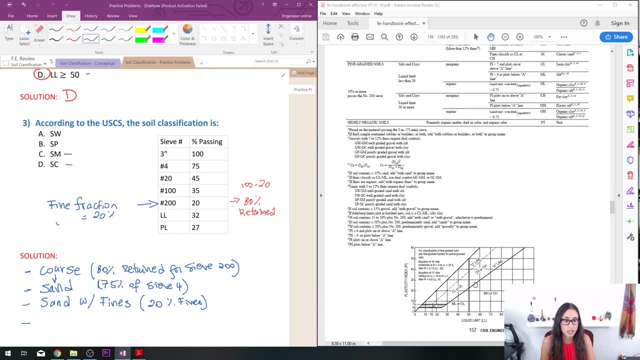 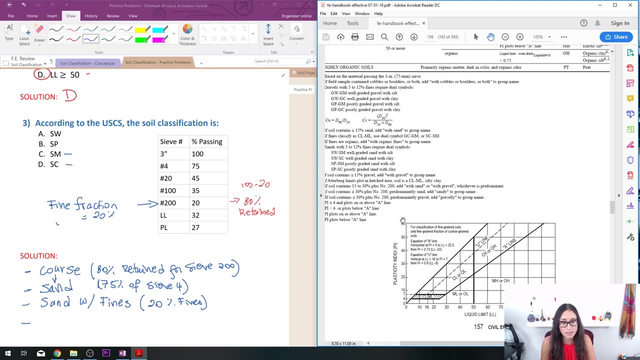 little bit tricky, but it's not that hard once you understand it. so we are going to go to our plasticity chart, which is down here, and what we're going to look at is our liquid limit and our plasticity index. now what was given to me is PL. right, I need to find my PI. so PI is just. 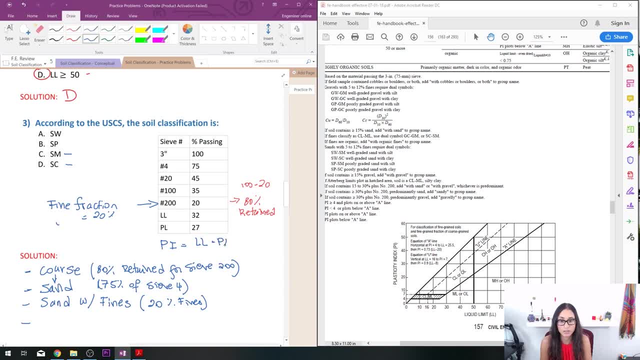 LL liquid limit minus PL. so that's going to be 32 minus 27: 5. okay, so with that, so I have 5 right here somewhere here, and then my, my liquid limit is 32, so I'm going to go here, which is somewhere here. so, on this area, as you can see, is all. 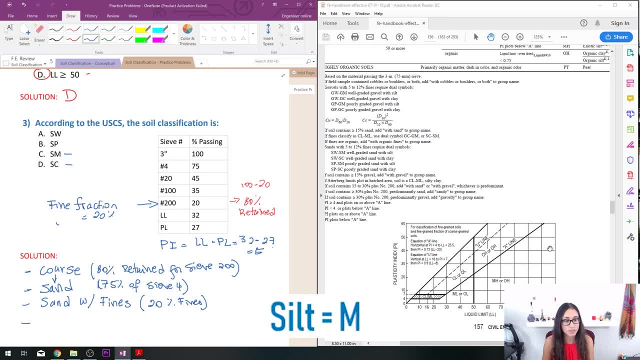 below a line, it's all silt. so I have n. so my answer is going to be SN, because I already defined it as sand with fines. I was just not sure if it was going to be silt or clay, but from this chart, because it's below a line, we can classify it as silty. 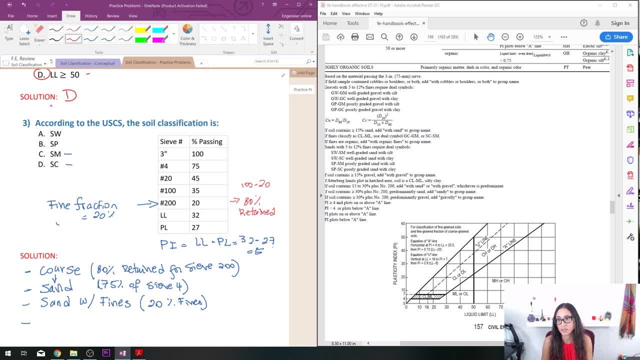 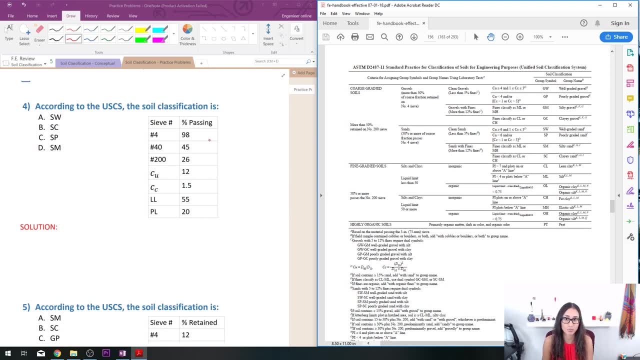 sand, so the answer is going to be C. next question- so we have the same question as before- is just different properties. so we have again here. we're going to always start with sieve number 20, because that's the one that defines your soil, either if it scores or it's fine. okay, so I have number 200. it's 26 percentage. 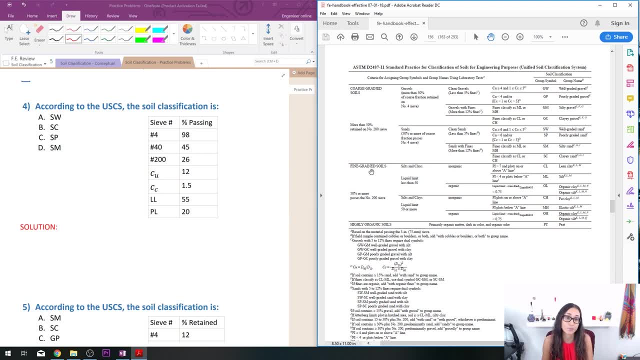 passing. so which means I have, it's gonna be this one, right, because more than 50% retained. and then here I have 26%, that's passing. here I need 50% or more. that needs to pass, sieve 200. so I'm going to say this: 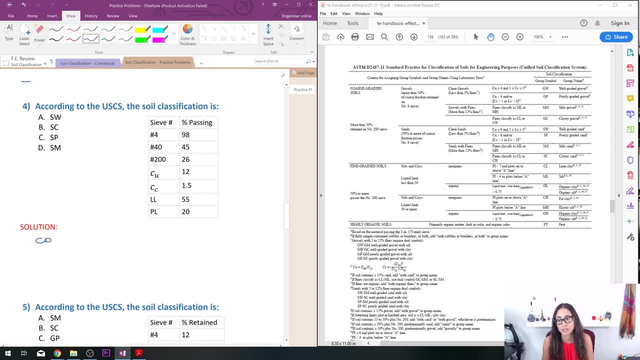 sole is going to be coarse. it's going to be coarse because I have 20%, 26% of sieve, 200, right, okay. next we're going to look at number four, sieve number four: so I have 98%. that passes my the sieve. so here I have 50% or more passing number. 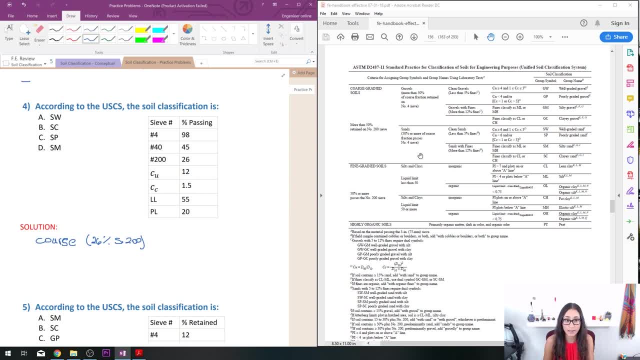 four. so it's going to be sand again. so I have sand because I have 40, I have 98% that passes. sieve four: now, after that, again, I need to define the, the, my fines. so my fine fraction this is: remember, this is your fine fraction. 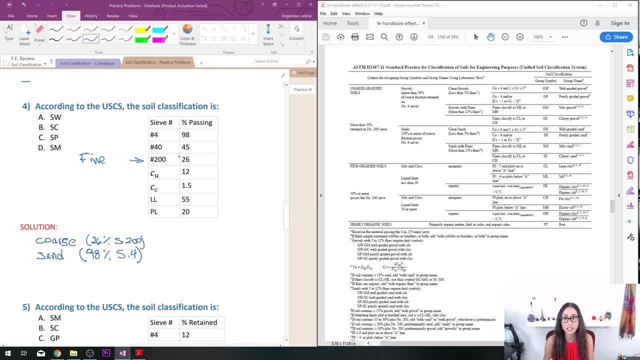 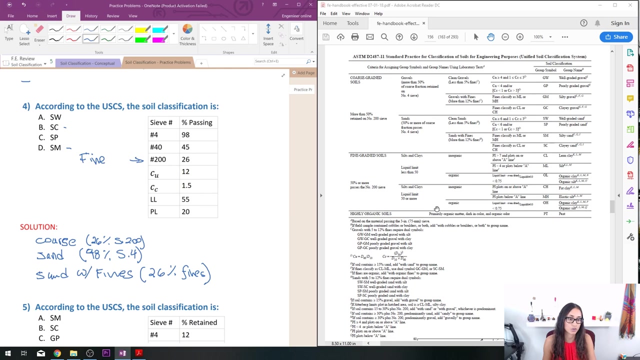 which is percentage passing of sieve 200. so that's going to be 26. now again it's more than 12%. so I have sand with fines and then that's because I have 26% fines. it's going to be either SM or SC. it's similar to earlier. 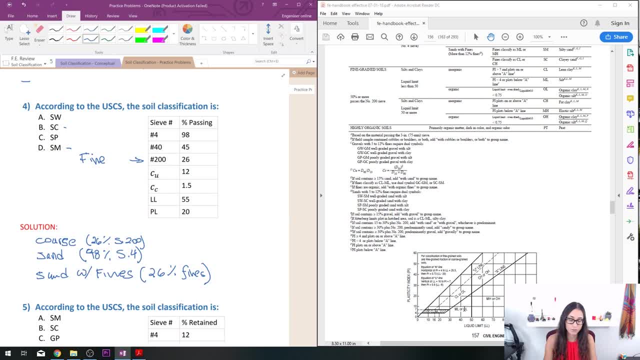 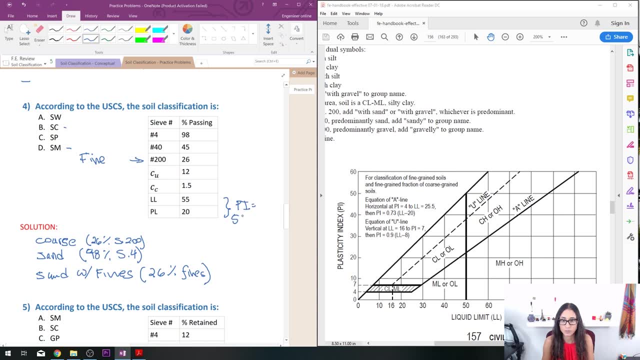 now we're going to come on to the chart so we need to find PI. so we said it's going to be 55 minus 20, which equals to 35. so my PI right here is 35. liquid limit is 55, which is about somewhere here. so this is above a line. so I'm going to have clay and 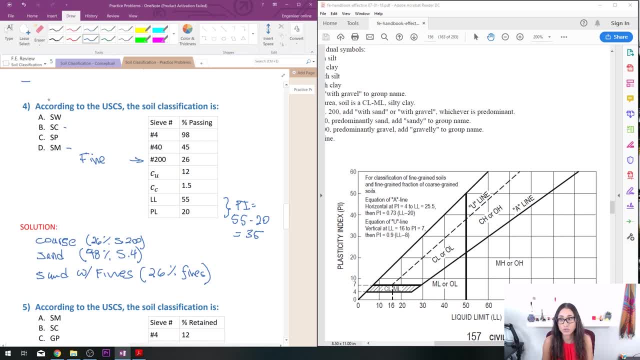 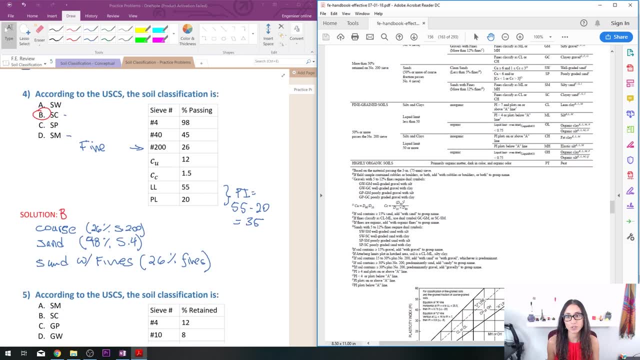 soil, so i have clay sand soil, so the answer is going to be sc and so that's b. notice, guys, here we didn't really use the uniformity coefficient or the gradation coefficient, so uh- or the seed number 40. so sometimes they do that in the test, they throw information that is extra that you 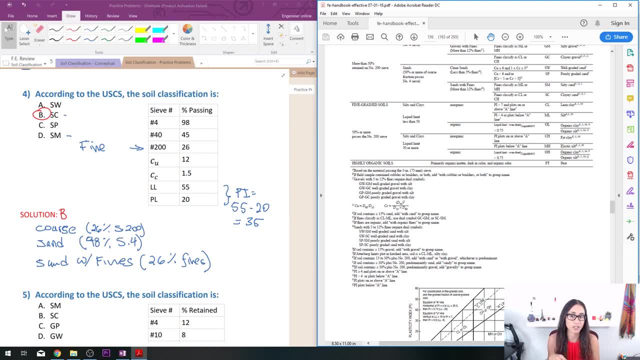 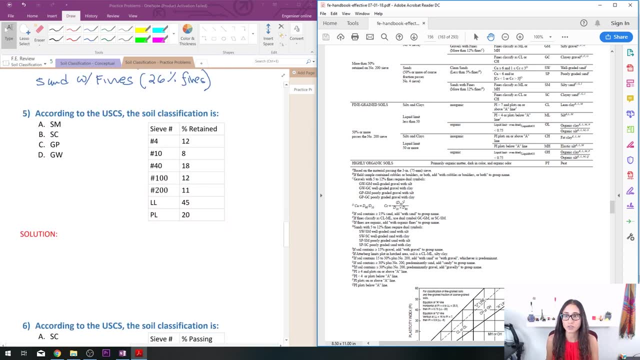 don't necessarily need. so, um, just be careful with that. and if you don't need to use it, you don't need to use it, so okay. so let's go to question number five. so, according to the uscs, the soil classification is sn, sc, gp or gw. now, this is very similar to the previous question that we had. 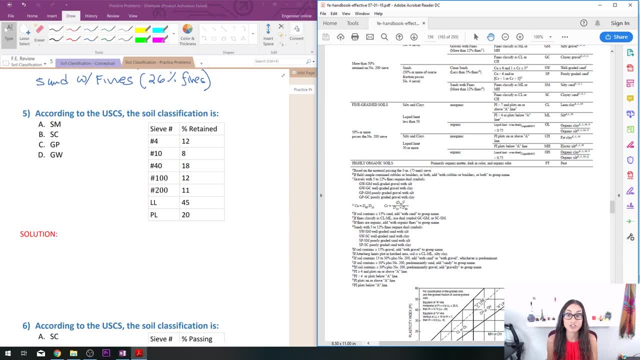 except this one. it gives you the percentage retained. so you got to be careful with this because, um, what you're going to need to do when you get percentage retained, we're going to actually need to sum up these uh percentages right here so that we can get number 200 c. so we're going to do so, let's. 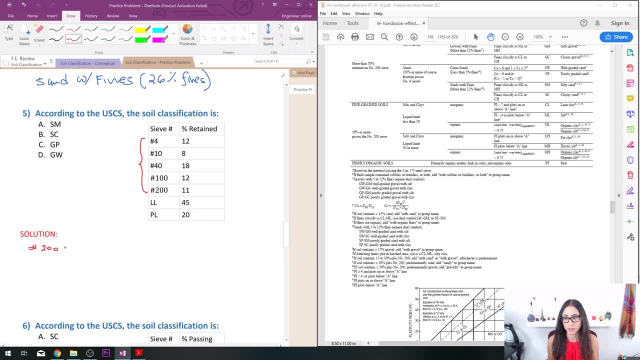 let's do it here. so number 200: it's going to be equals to 12 plus 8 plus 18 plus 12 plus 11, and that should give you a sum of 61. so this is your cumulative um retained percentage retained. so you have to actually do the sum so, or else you would get the 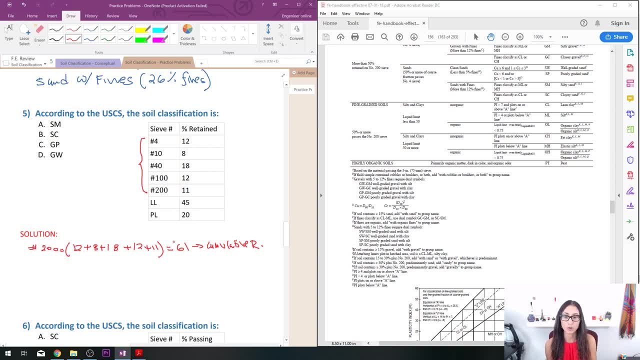 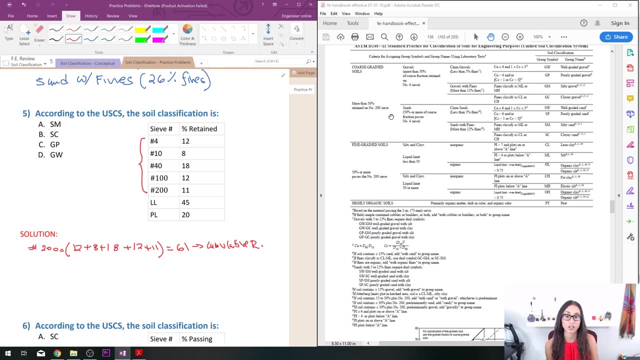 wrong answer. so if you want to know percentage passing, that will be 100 minus 61. okay, so with that information i have 61 percent. that is retained um in the seed number 200. so here i have more than 50 percent retained on 200, so which means i have coarse. 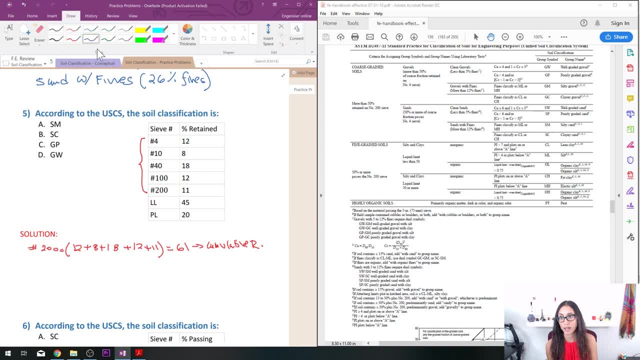 grain. so this classifies my soil as coarse grain. so if you just went with this number and you were like, okay, i have 11 percent retained, you are going to define it or classify it as fine grain and that's going to be a wrong answer. so make sure. 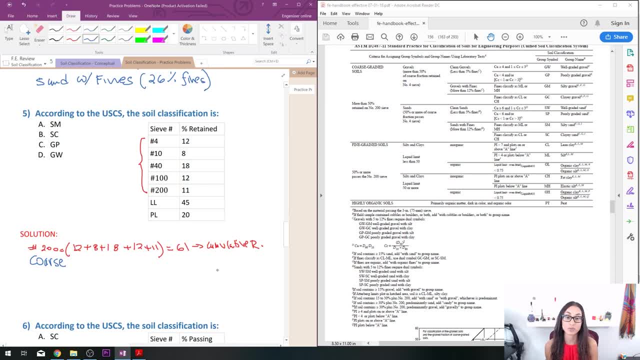 when you're giving percentage retained, you're going to have to need to do cumulative retained um percentage for you to be able to do that. so if you just went with this number and you were like 確usa a, you know, take 20 percent retained, you ever eventually verifood at 12 percent. 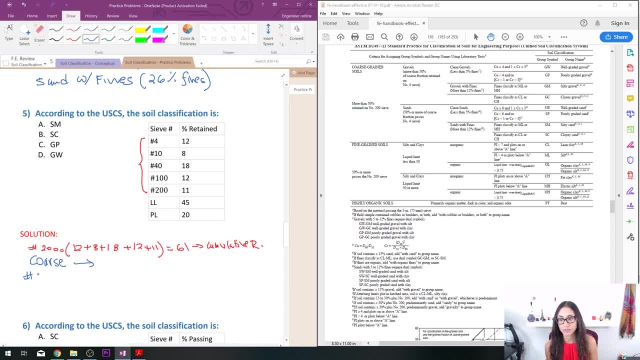 i'm told that it's from this 90 percent, like matthew testament, indicating that theאo no problem. so 40 percent retained for sure, and it's a point that we've justberries to be able to uh classify your soil, okay. so once we determined its cores again, then this is uh, we, we determined this to. 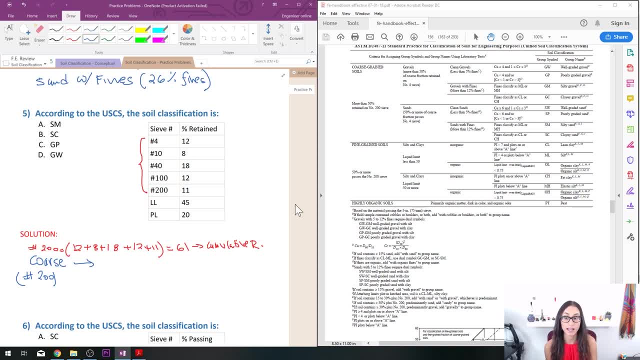 sieve 200. next thing we're going to look at is sieve number four. i have 12 percent retained, so sand. because I have only 12% that is retained, For it to be gravel I need more than 50% needs to be retained in sieve number four, So it's going to be classified as sand, So remember. 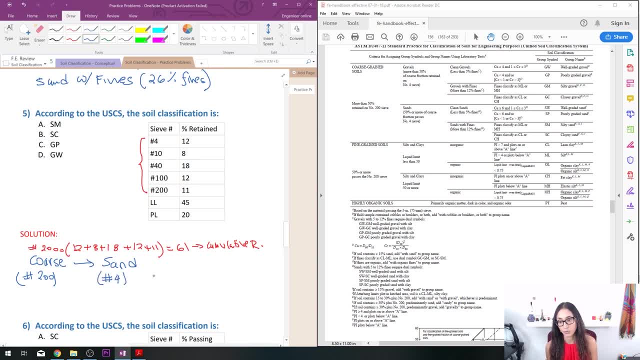 to classify as sand, we use sieve number four. Okay, the next thing we're going to do is find our finds again. Our find is the number, that is percentage passing, So we're going to have to actually calculate it. Find is going to be so the percentage retained: no, sorry. so the find is the. 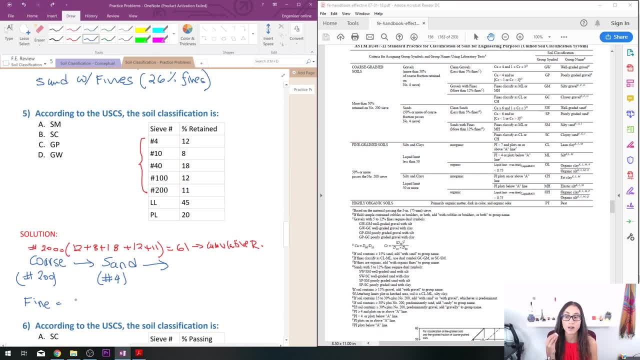 percent. oh yeah, the percentage passing through sieve 200, right, So? but then here I have 61% retained. So what I'm going to do is do 100 minus 61% that is retained, and this is going to give me 39% passing. 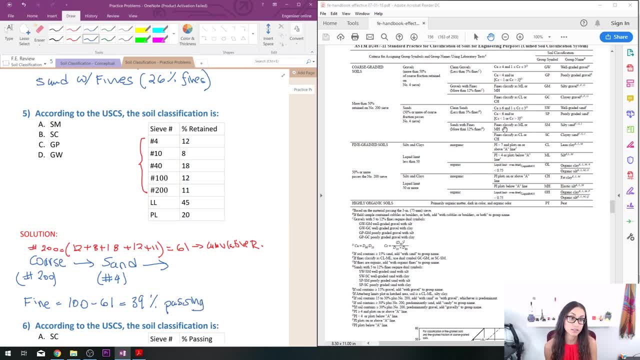 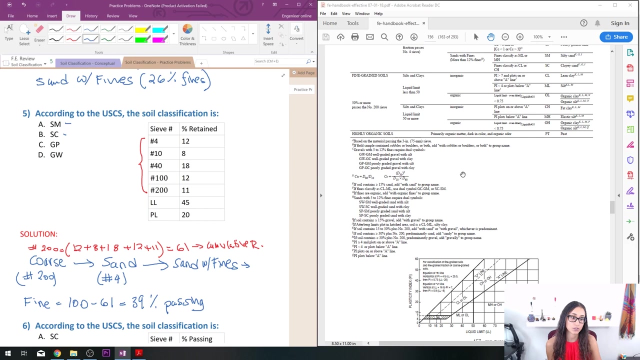 So I have more than 12% find. So again, I'm going to either classify it as sm or sc. Okay, so let's do sand with finds. Okay, So, as before, to determine if it's going to be silt or clay, we're going to need to look at the chart. 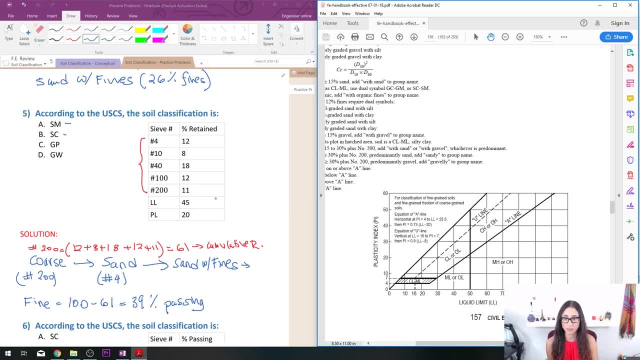 and then here I have: I need to find my liquid limit, Oh sorry, my plasticity index, pi, which is equal to liquid limit, minus plastic limit, which equals to 25.. Now liquid limit is 45, so somewhere here plasticity index is 25.. So it's going to be somewhere here. so it's above a line. So I have 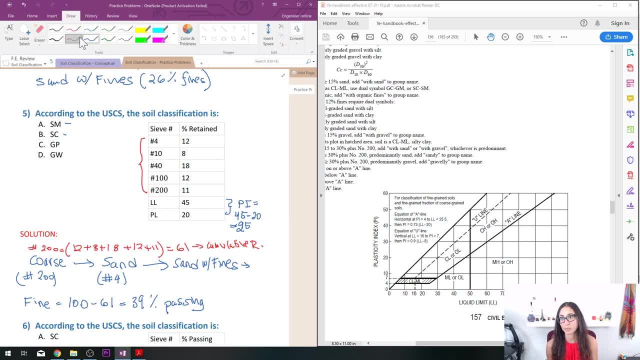 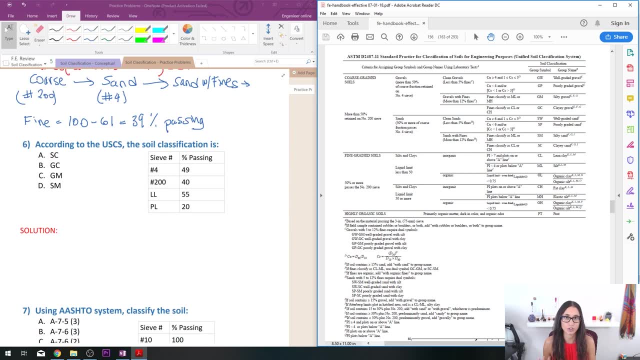 clay. so this. so my answer is going to be b sc, Question number six. This is the last question we're going to do about on new sc, as the next is going to be astro, But so the first thing we're going to look at is the. 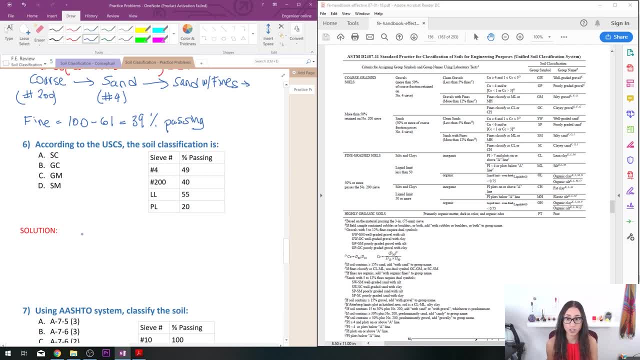 percentage passing for sieve number 200. So I have 40, which means it's going to be coarse, Right, because 50% or more passes number 200 is fine grained. I have only 40. So that's going to be coarse. After that we're going to look at sieve number four. So I have 49% passing. 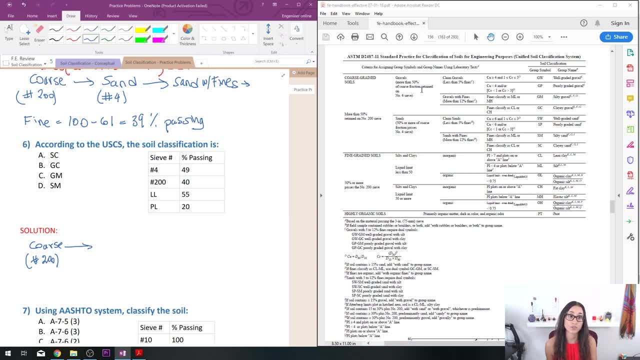 So that puts me into. so I have more than 50% retained and I have 50% or more. that passes number four. I only have 49. So that's going to be gravel. Then we're going to look at the fine percentage which is, for our case, is 40. So this is your fine. 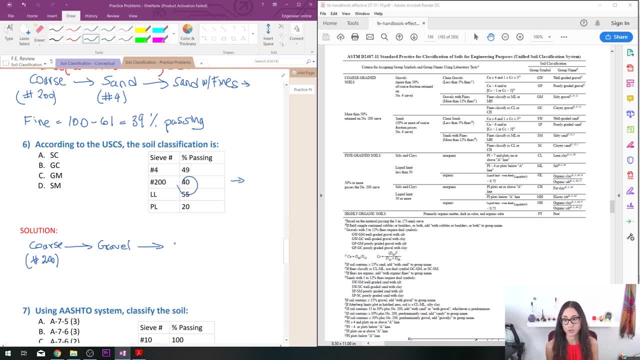 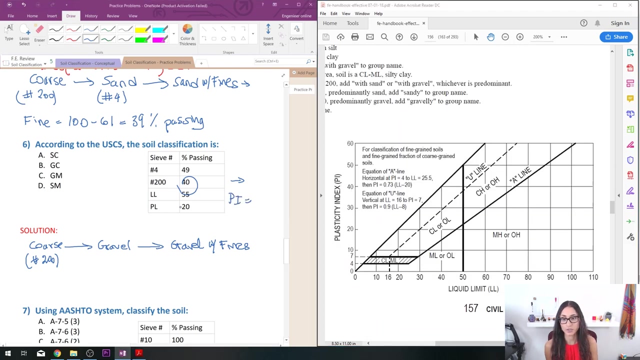 is 40. So more than 12%. So I'm going to have gravel With fines. Then the next thing we're going to look at is: is it silt or is it clay? To determine that, we look at the table first. calculate pi, which is 55 minus 20, which gives you 35. So I have 35. 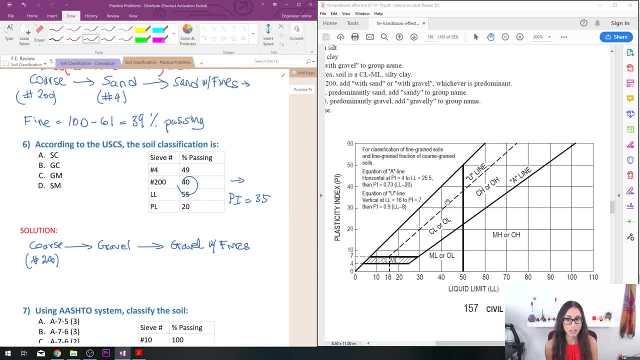 pi, which is somewhere here. then I have my liquid limit at 55,, which is somewhere here. liquid limit at 55,, which is somewhere here. then I have my liquid limit at 55,, which is somewhere here. then I have my liquid limit at 55,, which is somewhere. 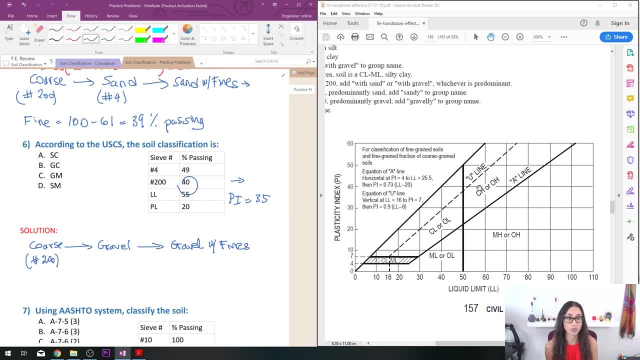 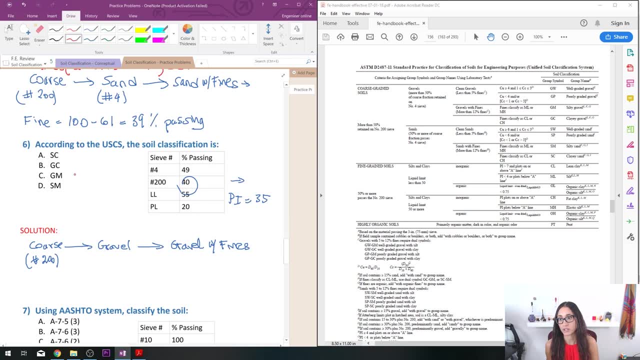 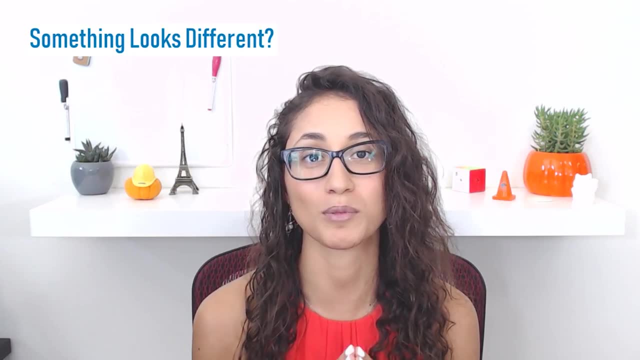 here. so it's above a line, so it's going to be clay. so we said clay, so it's going to be gc, which is b. so that's my answer. my answer is b. okay, guys, so the last problem we're going to cover here is problem number six, because the original video was a little bit too long and i like to keep my. 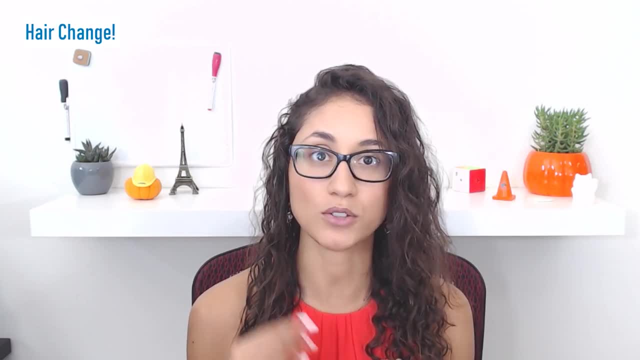 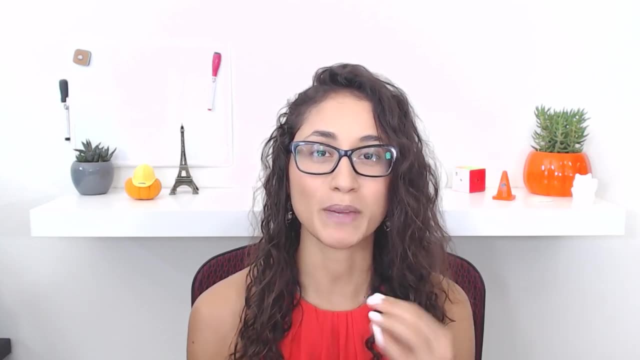 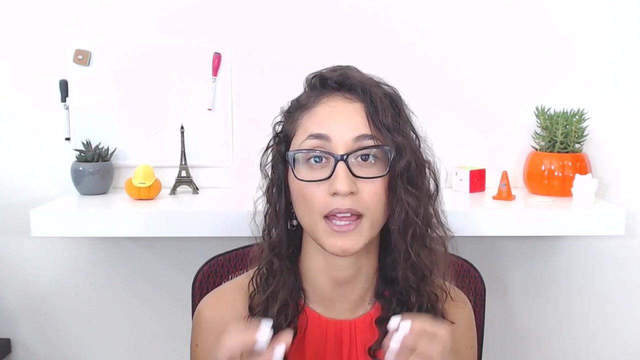 videos under 20 to 25 minutes. that way you don't get bored or discouraged, and also it gives you enough time to grasp and understand the material. now make sure you try to do these problems with me as you go, because the best way to learn something is by doing it and practicing a lot. so keep that. 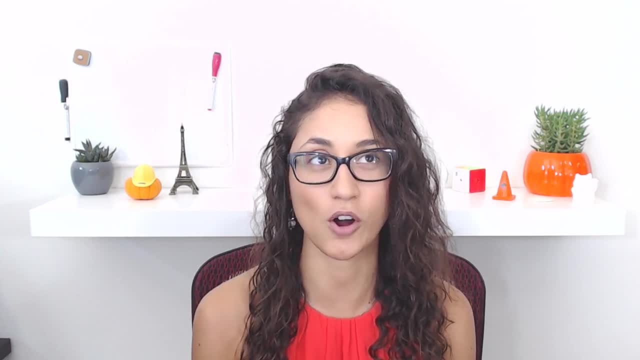 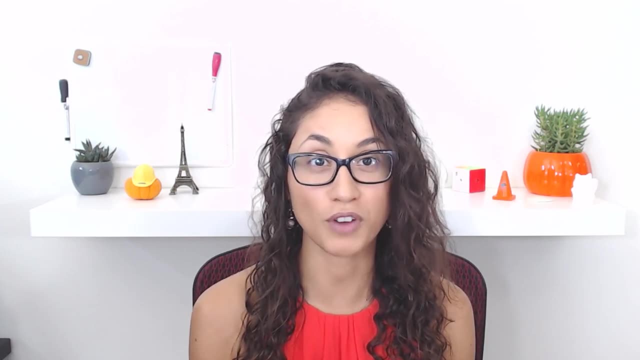 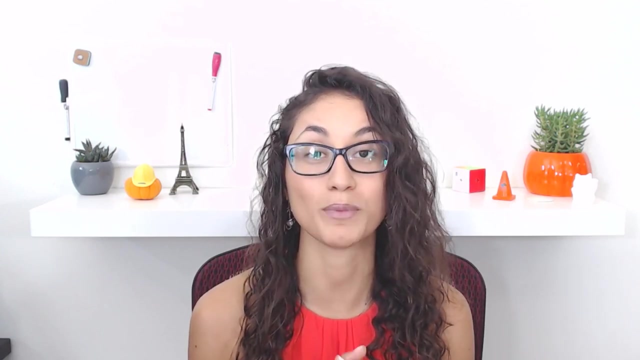 in mind, and don't forget to watch the second part of this video, where we cover problems using ash. and in the fe exam, or the midterm or your final in soil mechanics, you may ask to classify the soil using both methods or one of them. so make sure you know both of them, and we're going to also end the video with the homework. 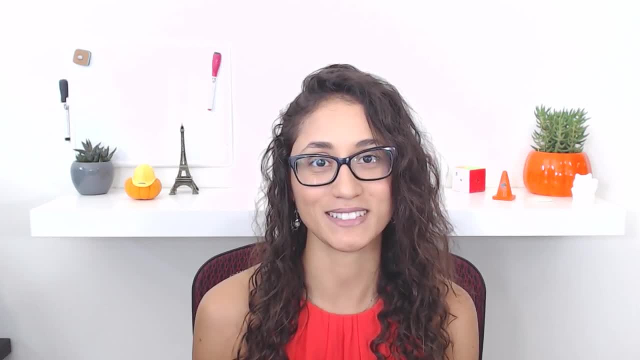 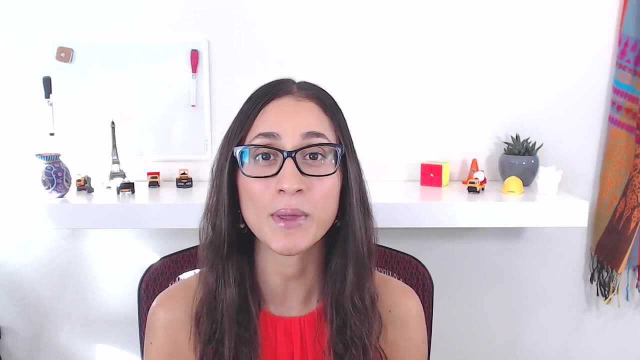 problem for you to attempt at home, so you don't want to miss it. so i tried to go over problems that are a little bit tricky. hopefully that can help you tackle any problem that you get in your fe exam. now, if you have any question or is there a specific problem that you would like me to go over, 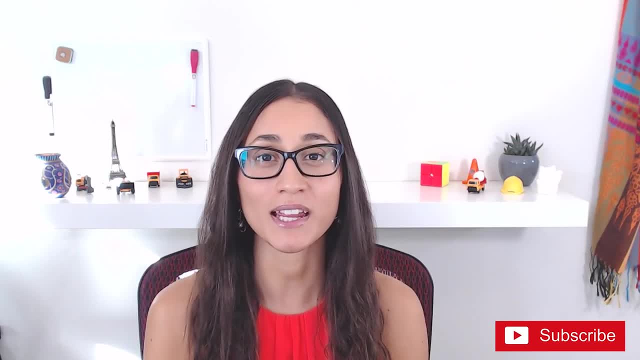 please leave it in the comments below. don't forget to subscribe, like and make sure to share with your friends who might find it helpful. thank you, guys for watching and i will see you soon. see you next time.